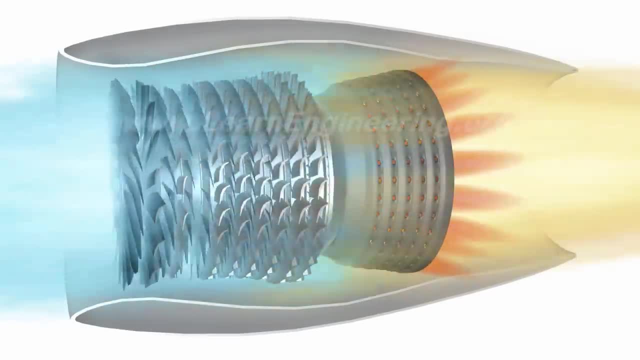 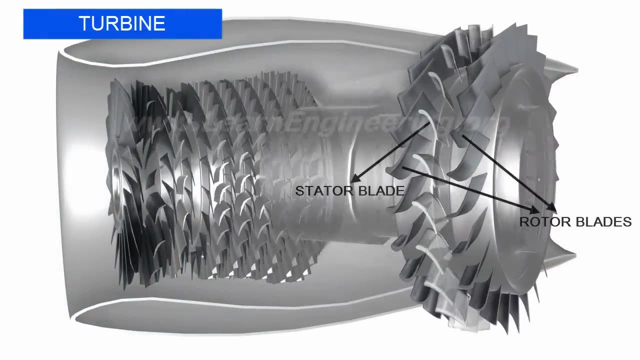 The compressor receives the air from the air pump and the air is released into the air pump. The air pump receives the energy for the rotation from a turbine which is placed right after the combustion chamber. The compressor and turbine are attached to the same shaft. 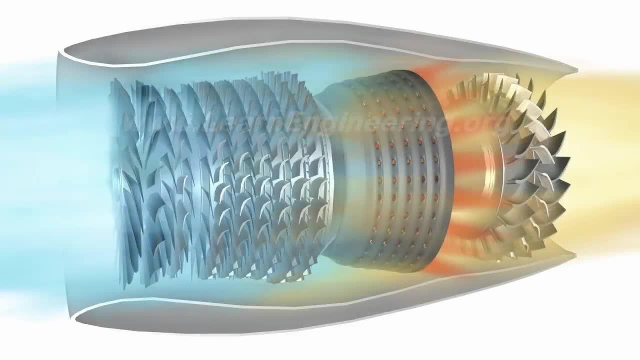 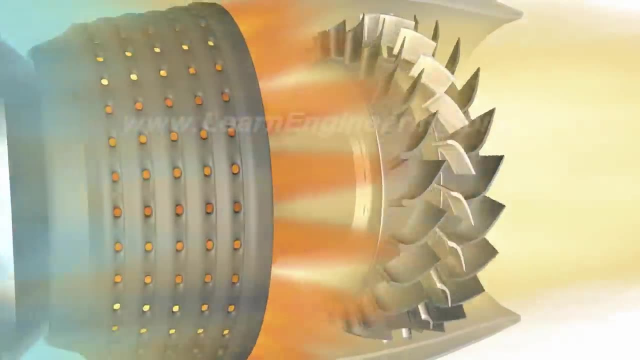 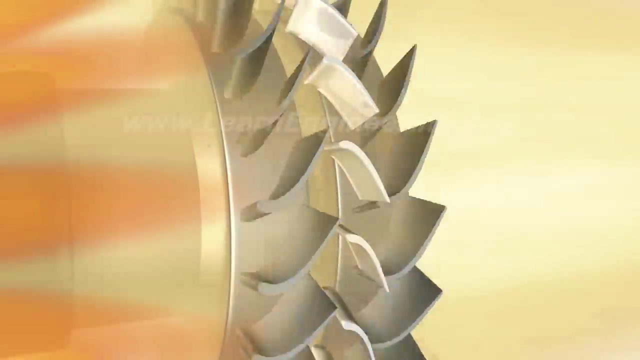 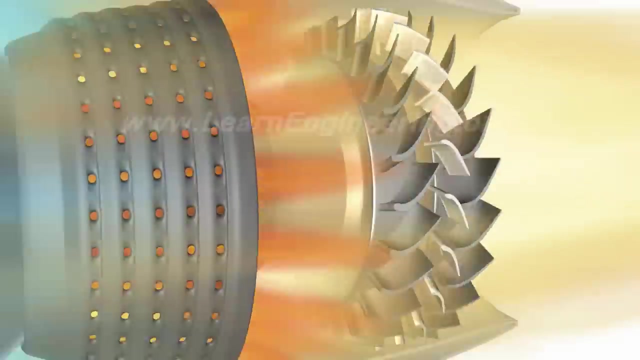 The high-energy fluid that leaves the chamber makes the turbine blades turn. You can see that the turbine blades have a special airfoil shape, which creates lift force and make them turn. As the turbine absorbs energy from the fluid, its pressure drops. Through these steps we 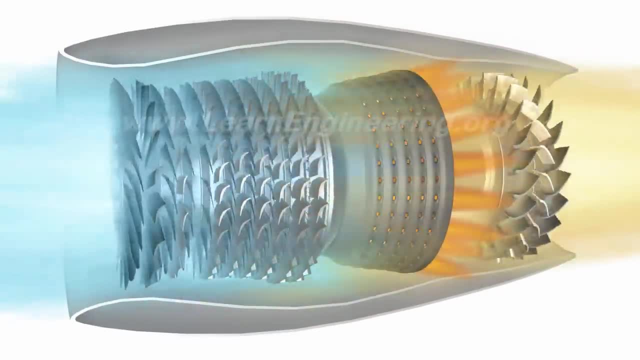 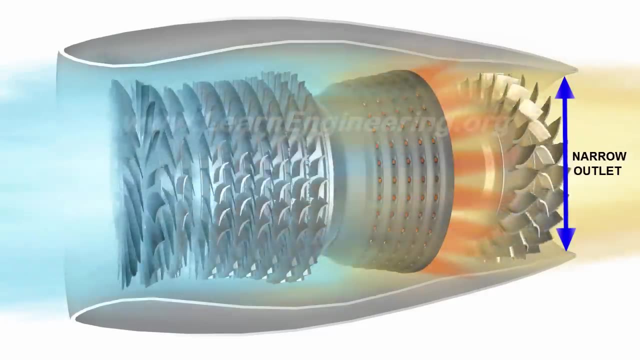 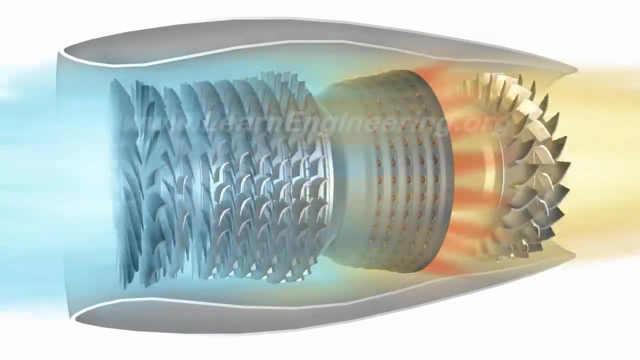 have achieved our objective: a really hot and high-speed air emitted from the exit of the engine. The engine case becomes narrower towards the outlet, which results in even greater jet velocity. In short, the synchronized operation of the compressor, combustion chamber and turbine makes the aircraft move forward. 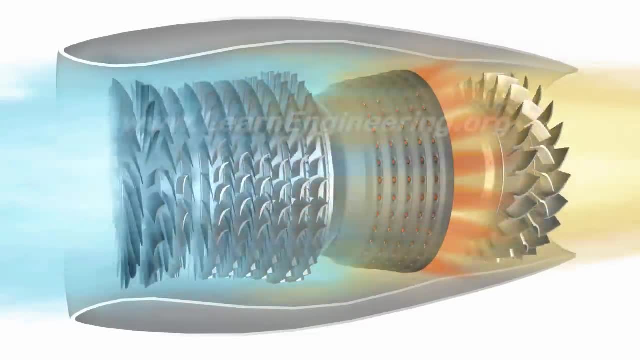 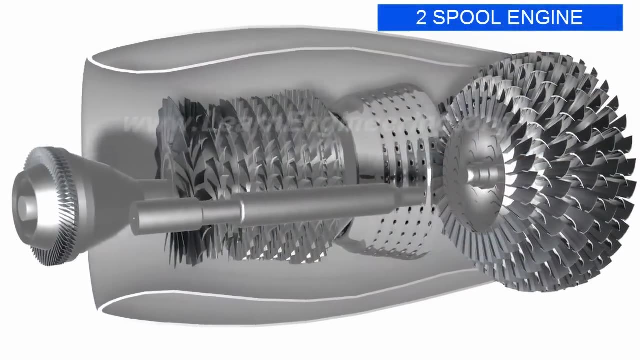 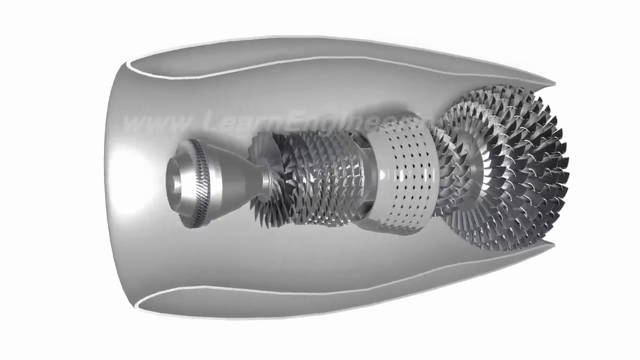 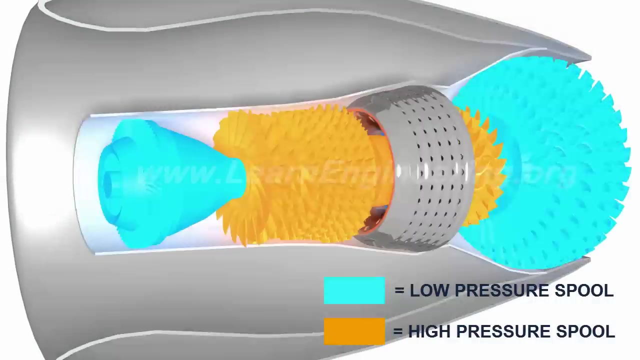 Modern aircrafts use a slightly improved compressor turbine arrangement called a two-spool. Here two independent turbine compressor stages are used. The shaft of the outer compressor turbine passes concentrically through the inner one. The outer turbine is subjected a low energy fluid and will run at a lower speed than the inner turbine. 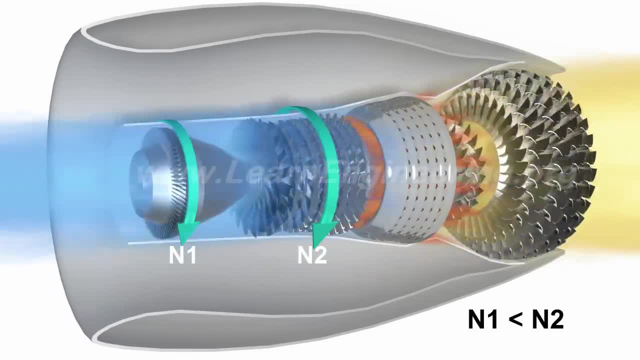 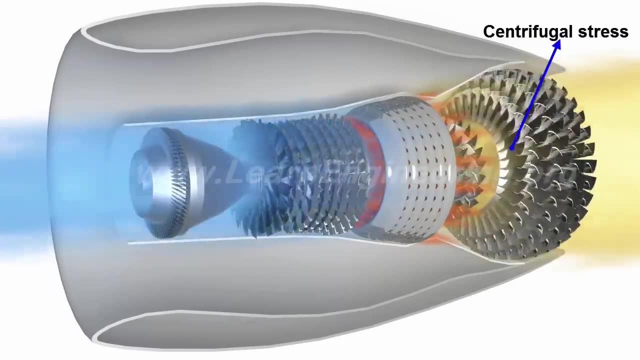 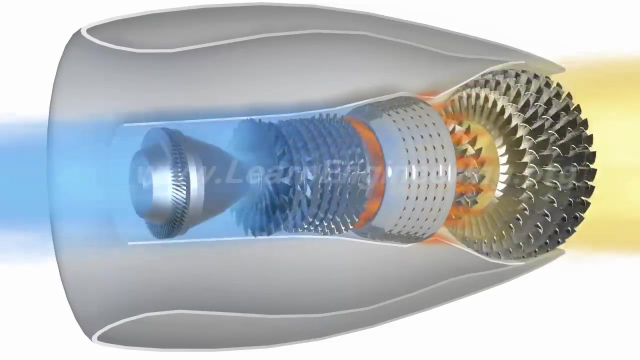 Low pressure blades are longer. This low speed helps to reduce centrifugal stress induced at the root, thus improving the blade's life. Some modern aircrafts even use a three spool engine. The engine we have discussed so far is more specifically called as: 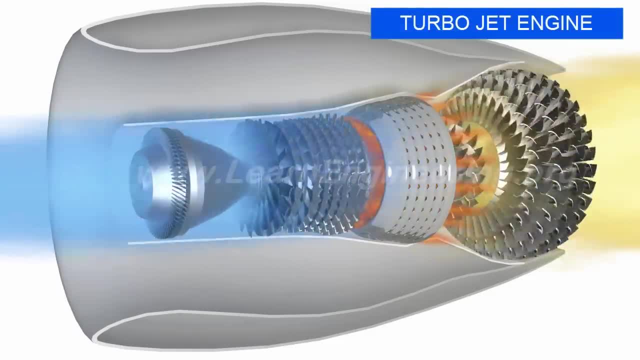 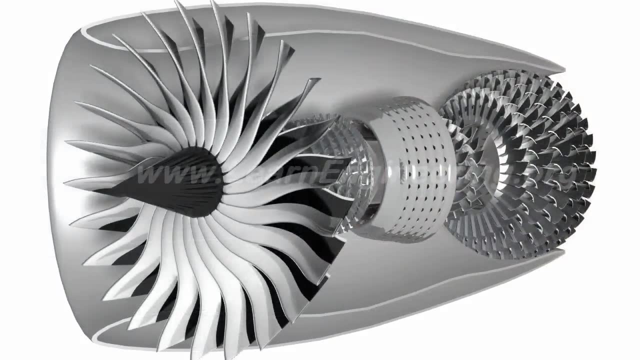 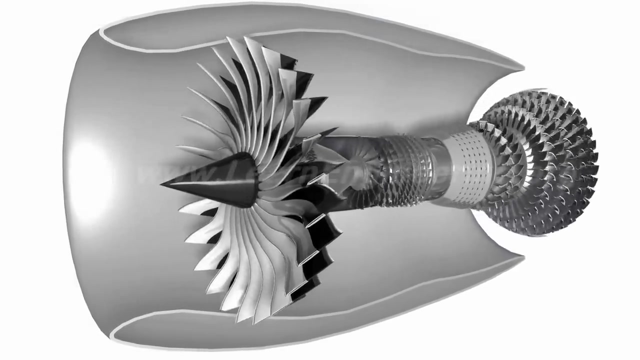 turbojet engine. Turbojet engines tend to produce high levels of noise, like air稼a and steam air. A revolutionary improvement was made to this engine by fitting a large fan with the low pressure spool. Such engines are called turbofan engines and almost every commercial aircraft run on them.